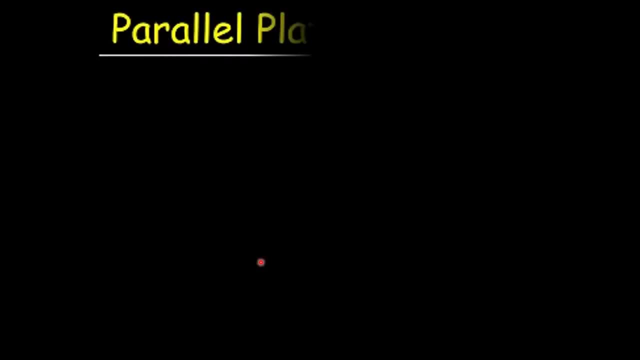 Dear students, in this video lecture we are going to discuss about a parallel plate capacitor. Dear students, capacitor is a device which is used to store electrical energy. Electrical energy is stored in a form of charge, So we can define capacitor as capacitor is a device which stores electrical energy in a form of charge. 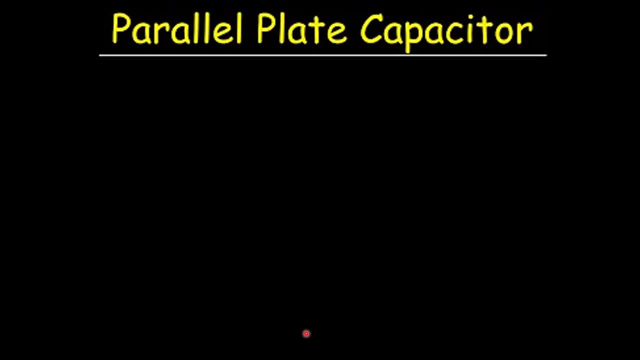 Capacitor consists of two plates. Capacitor consists of two plates And these two plates are conductors, So the conductor of capacitor. Basically, they store charges And these electrical charges basically cause a creation of a potential difference between the plate of the capacitor. 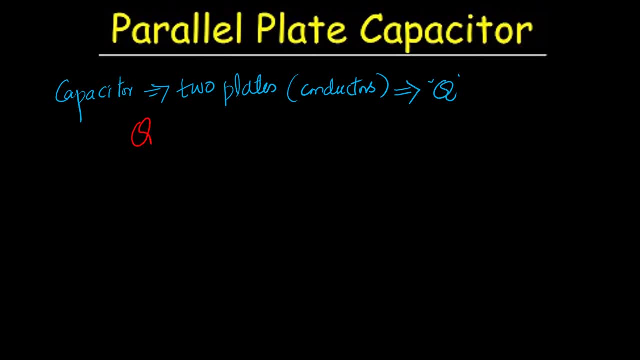 So we can write that the charge stored in a plate of a capacitor is directly proportional to the potential difference between the two plates. So we can open this equation And, as Q is equal to constant, into V, V is a potential difference. 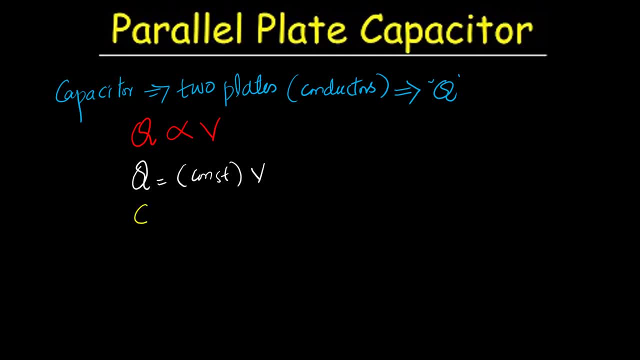 So the unit of constant is represented by C, which is known as capacitance of a capacitor. The capacitance of a capacitor is a ratio of charge stored In a plate of a capacitor by a potential difference created between the plate of the capacitors. 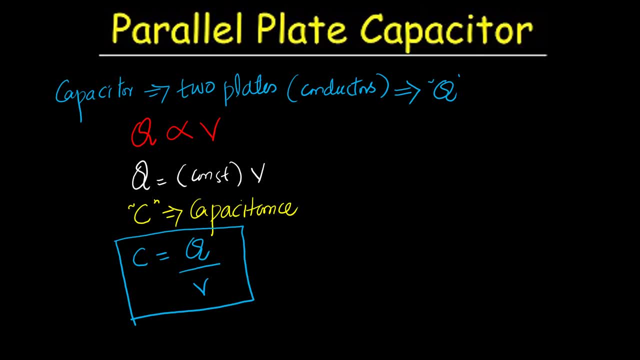 So we can define capacitance of a capacitor, as capacitance of a capacitor is ability of a capacitor. It is the ability of a capacitor To store electric charges. The unit of capacitance of a capacitor is known as Farad, And since you know that, C 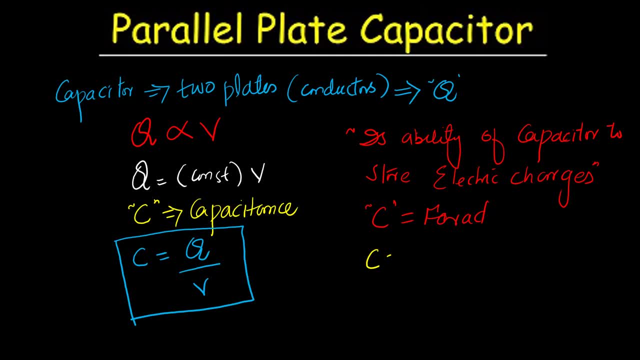 Since you know that capacitance is a ratio of charge, It is the ability of a capacitor to store electric charges. So we can write that the charge stored divided by a potential difference. So the unit of charge is C, Whereas the unit of potential difference is V. 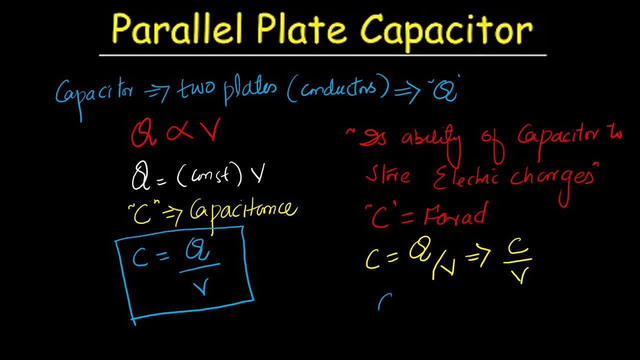 So the SI unit for a capacitance of a capacitor is C per V And it is also written as Farad, So the unit of capacitance of a capacitor is Farad. So the unit of capacitance of a capacitor is V. 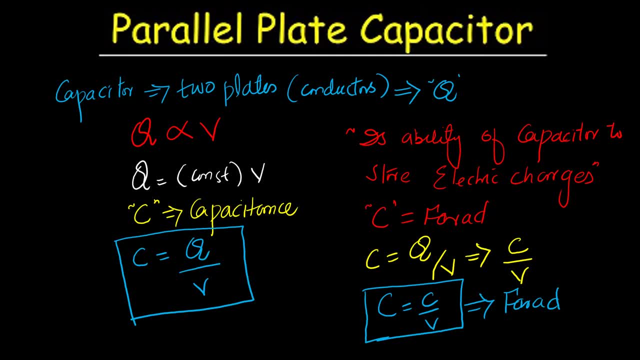 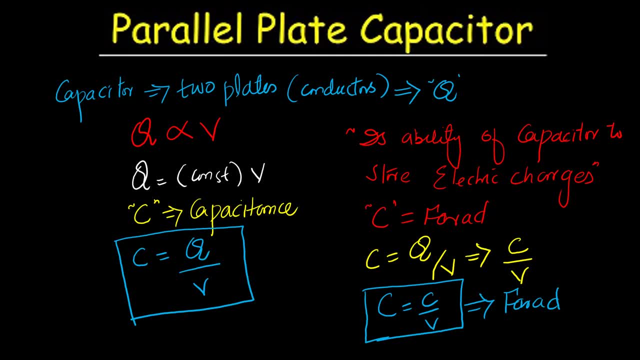 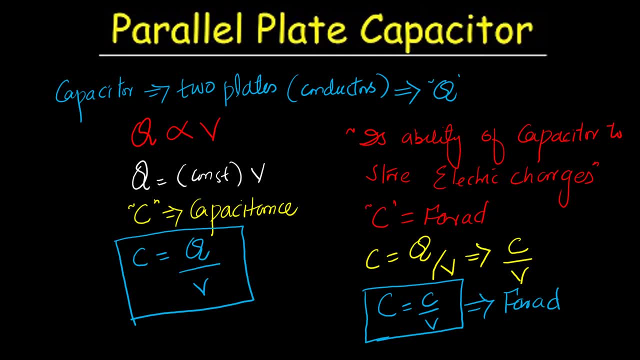 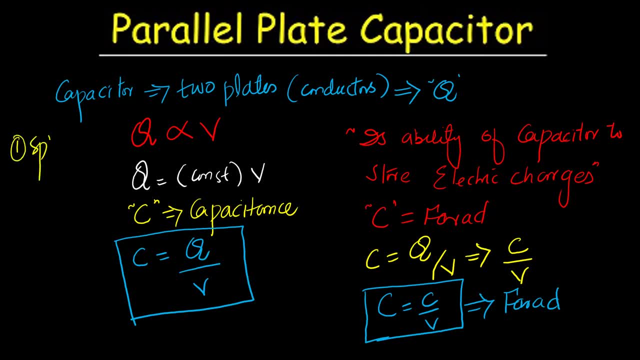 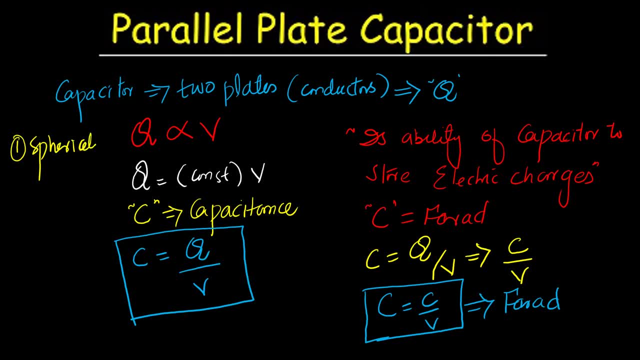 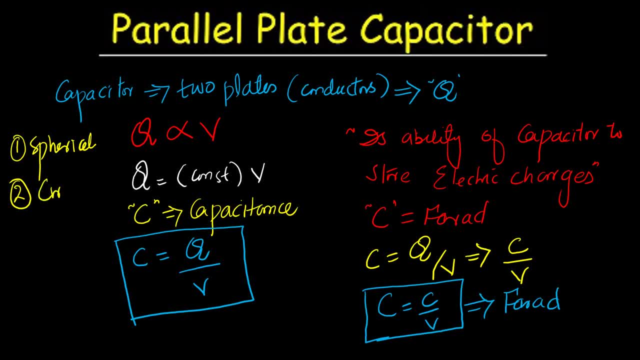 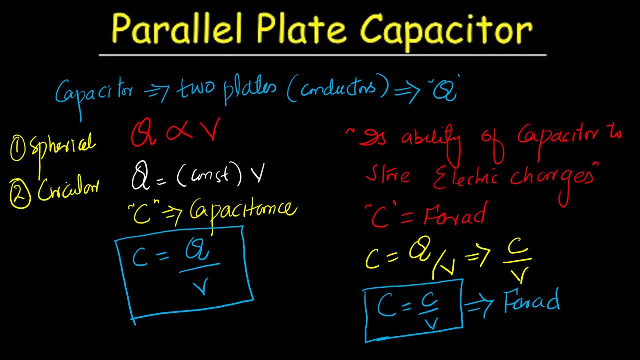 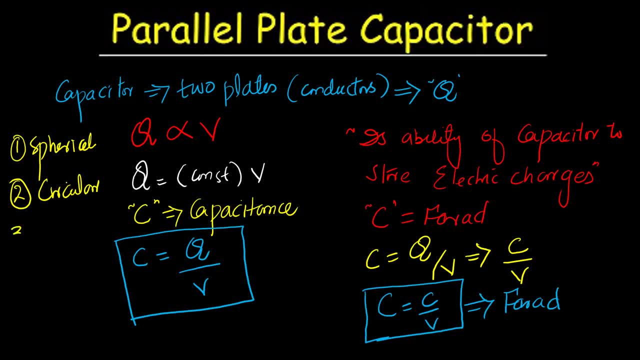 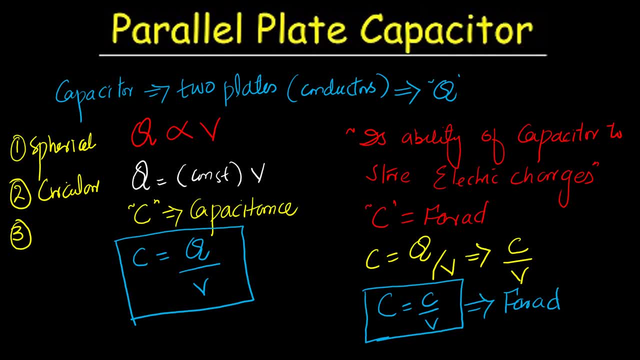 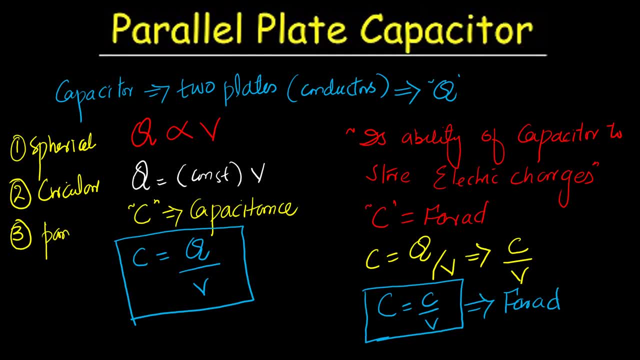 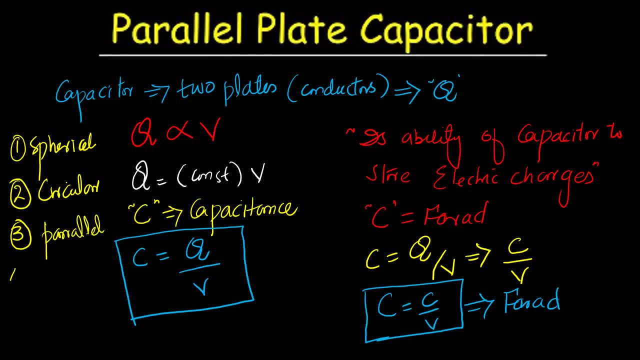 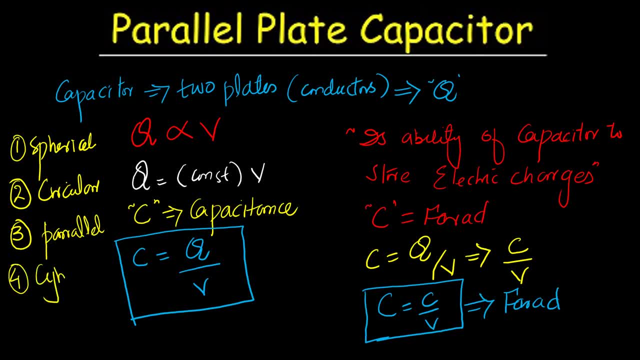 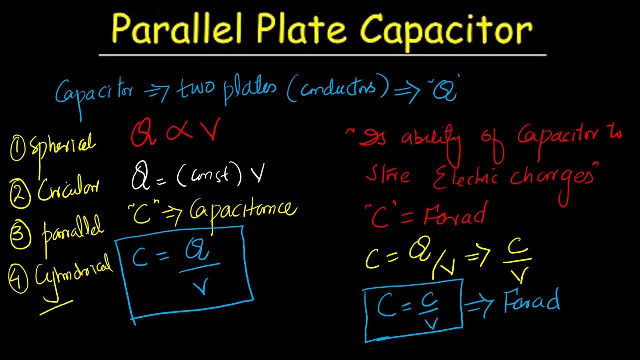 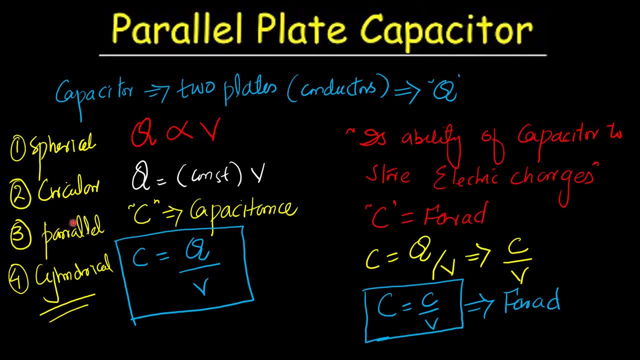 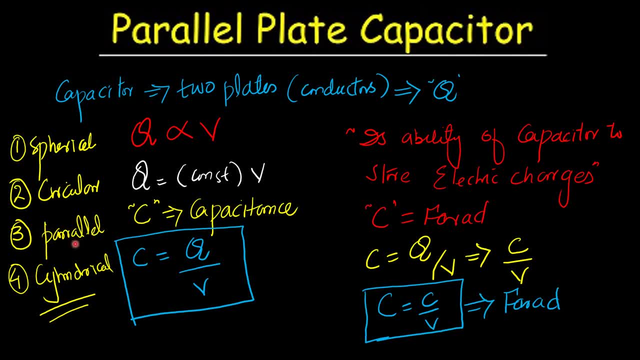 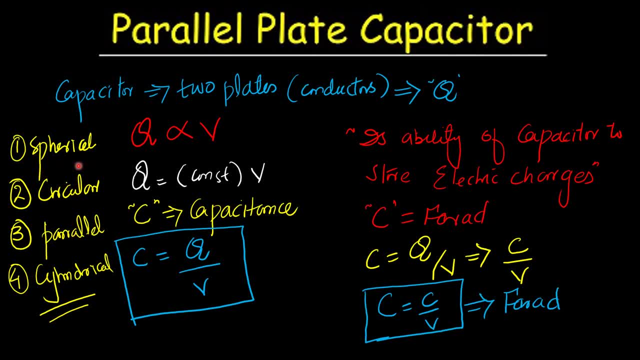 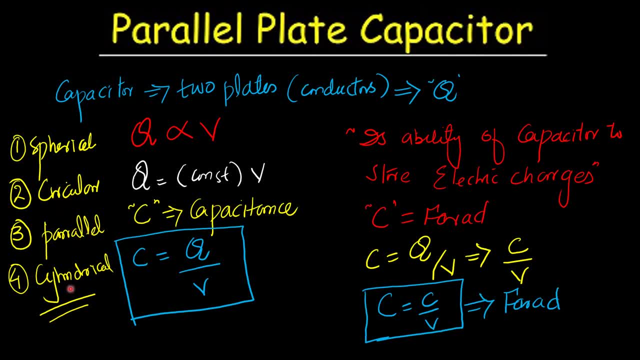 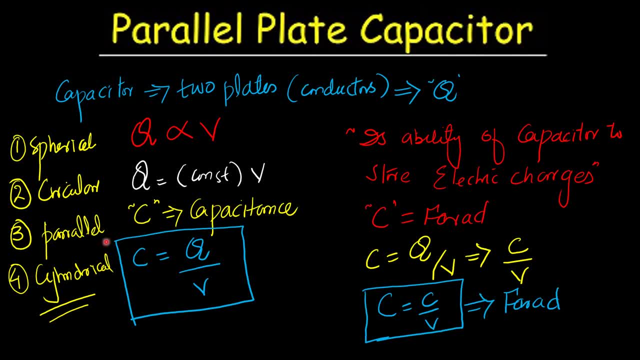 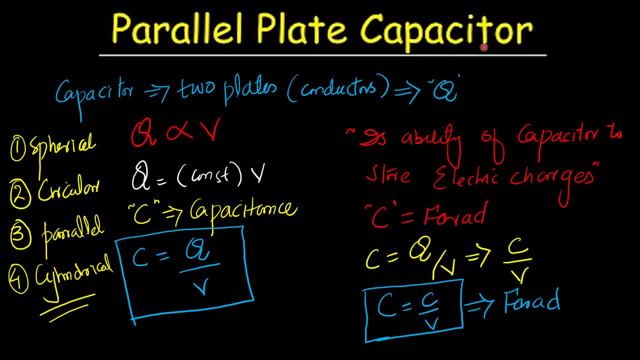 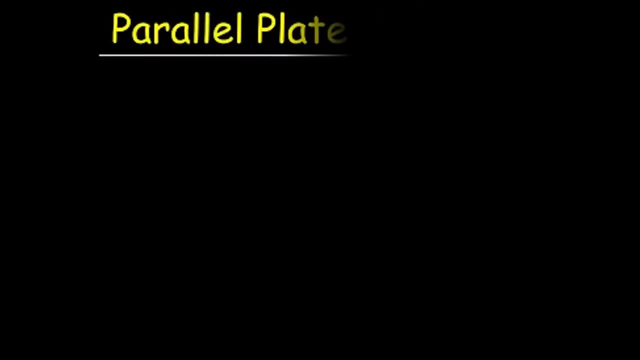 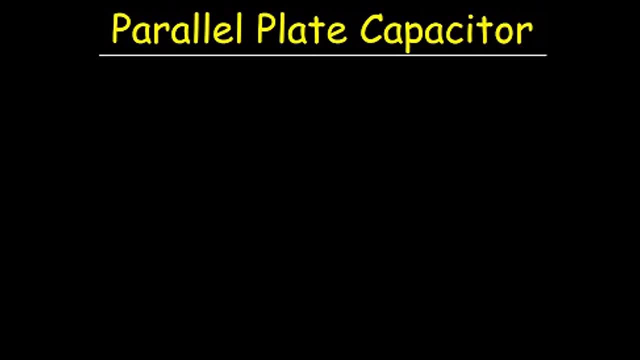 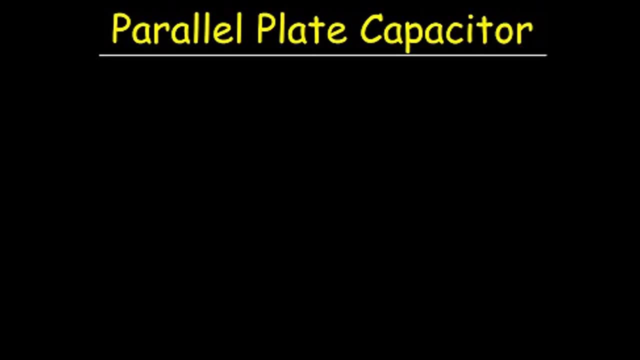 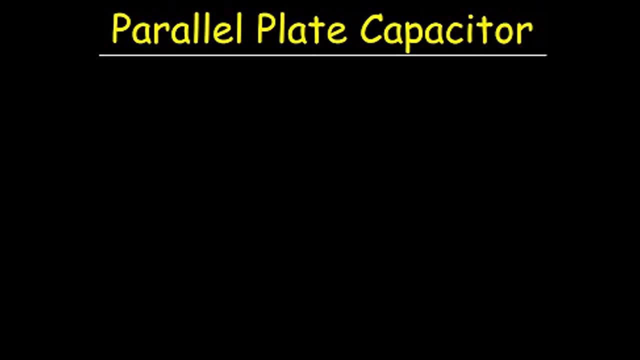 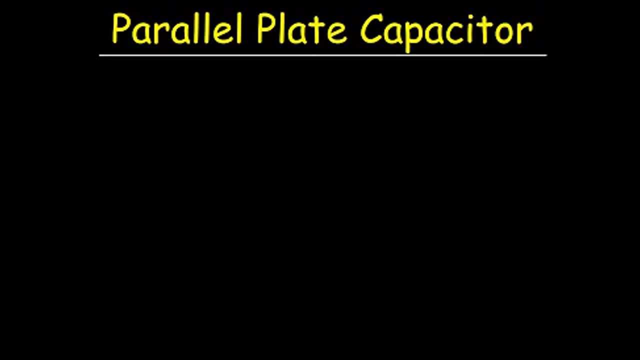 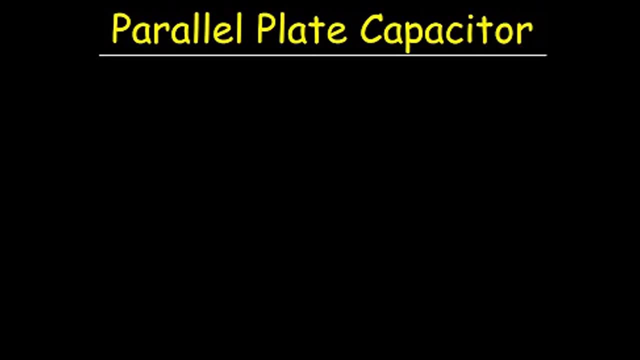 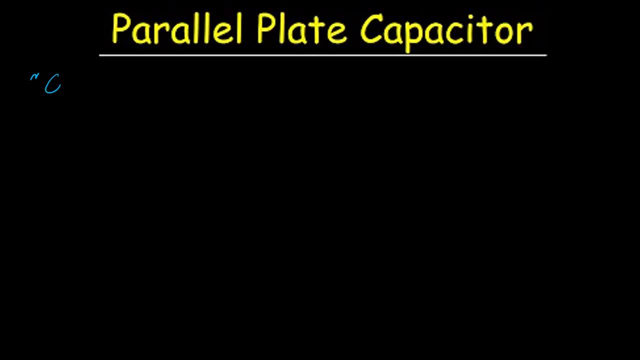 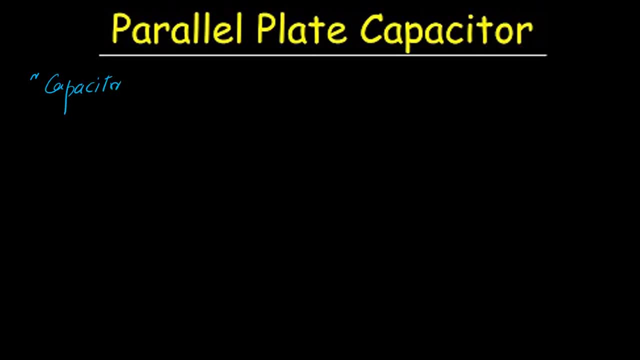 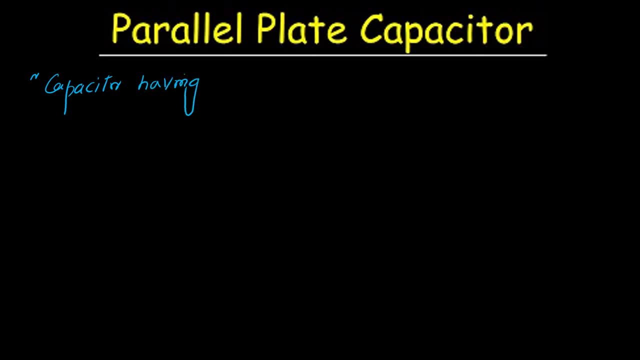 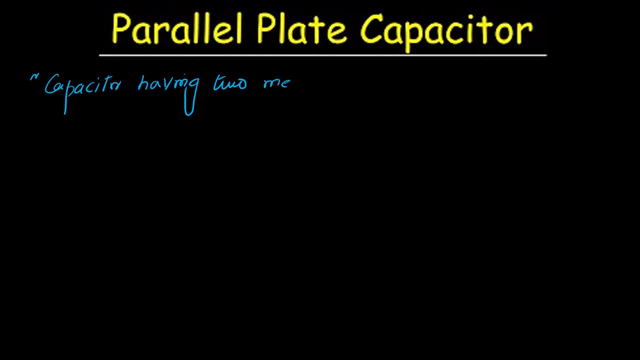 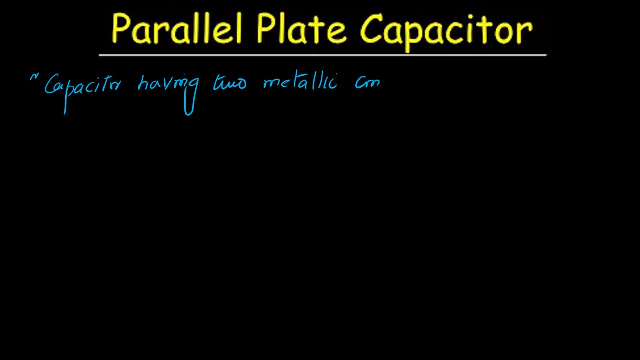 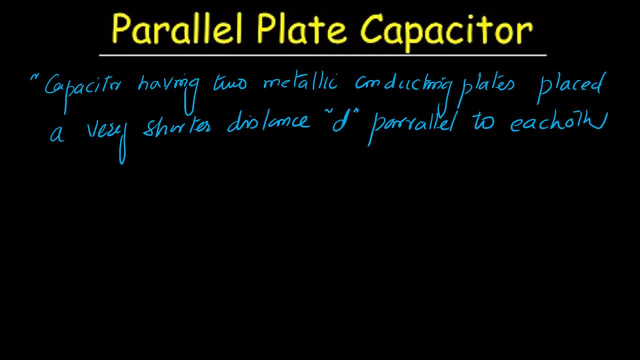 So we can represent the parallel plate capacitor with a schematic diagram. Basically these are two parallel plates. Suppose this is a parallel conducting plate S1 and S2, this is another conducting plate, S2, and both these plates are basically placed parallel to each other due to this. 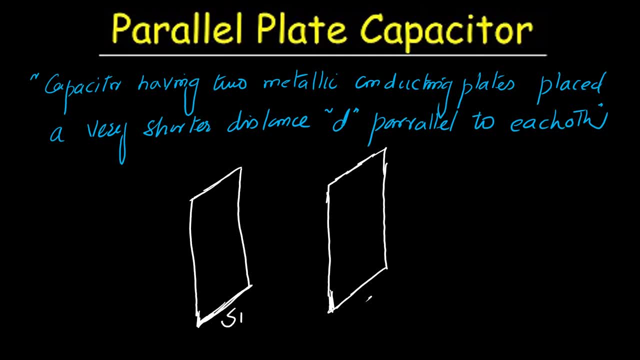 The charges are stored in these parallel plates And, due to this, the position or the placement of the plates in the capacitor. these capacitors are known as parallel plate capacitors. Students, please keep in mind that the area of the plates of the parallel plate capacitor is always same. 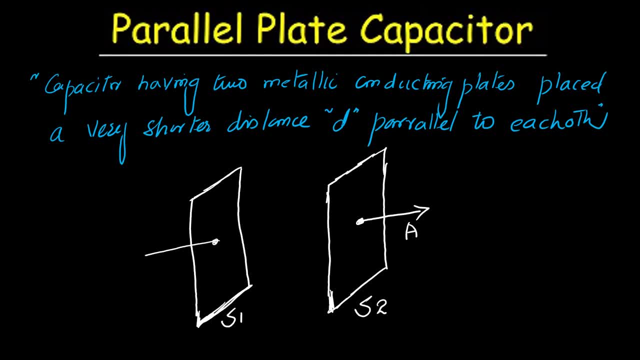 It is area vector for both the parallel plates of the parallel plate capacitors is same, So it is a property of parallel-proof capacitor. First, the area of the parallel plate capacitor is same, Area of plates of capacitors is same. And second, property of the parallel plate capacitor is that 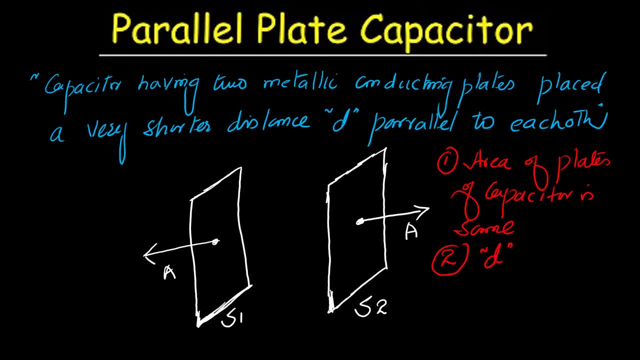 the spacing, the space or a distance between which is we represent here with a D. The space between a parallel plate. D is very small, is very small than the area of plate area of plates. So D will be very, very, very small than the area of the plates. 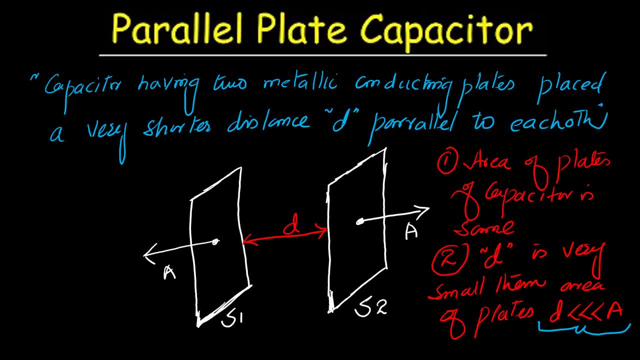 And due to this, we can say that area D is appear as nearly area, We can say that area A appear nearly infinite, infinite for the, for the, for the space or distance, or a distance between two parallel plates. Because- and this that is the reason if this- 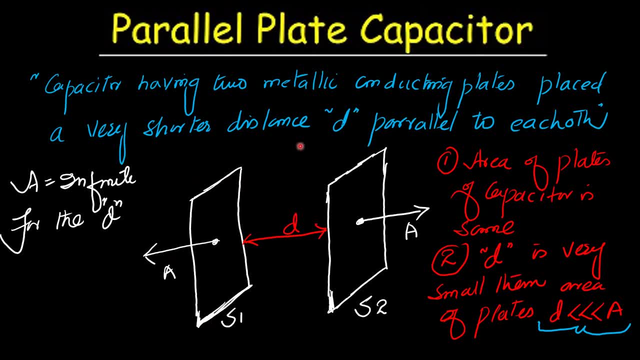 if the distance between D, between these two parallel plate, is larger than there will be, efficiency of the capacitor will decrease because the electric field of reliance cannot basically interact across these two plates or the storage will be difficult. So, in order to get an efficient capacitor, 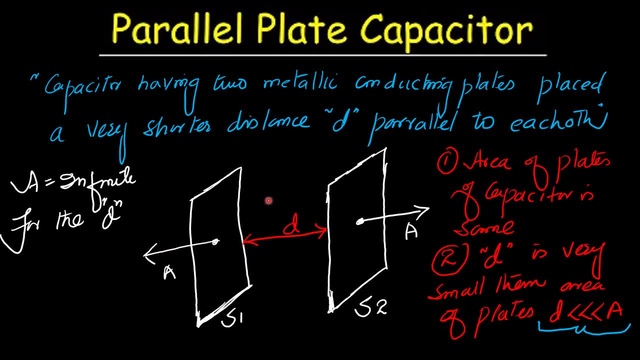 the distance between the two parallel plates. parallel plate is very small and it is nearly negligible to the area of the plates. This student please keep in mind that electric field of lines. suppose that in one plate there will be in parallel plate capacitor there will be a positive Q charge. and where as when? 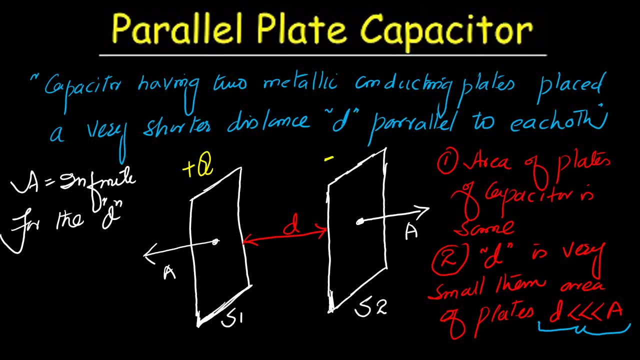 the charge is stored in them and on other plate there will be a negative Q charge and you know that the electric field of line basically they electric field of line. they basically move from positive charge towards a negative charge. these are electric field of lines. they basically are directed from positive charge towards the negative charge. 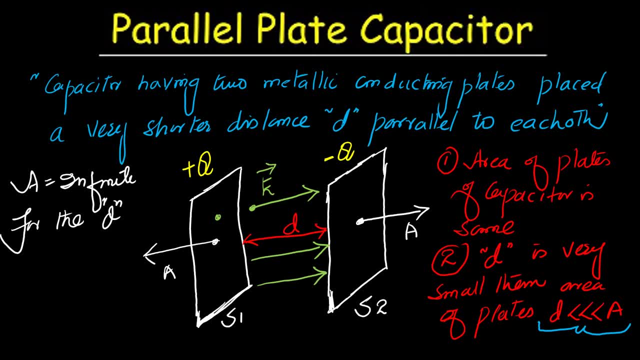 So in parallel plate capacitor, the electric field of lines. electric field of lines is the third condition. in parallel plate capacitor, the electric field of lines are bounded, Bounded from positive charge to negative charge of the plate. So this student, please keep in mind that if, if the space D is less, less, less than area, 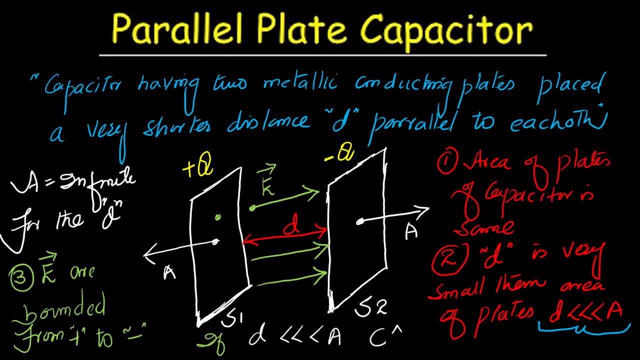 than the capacitor, Then the distance of the capacitor will be more. So from here we can say that the capacitance of a capacitor depend on a distance between a parallel plate and as well as area of a parallel plate. This mean that capacitance will be greater if the distance between the plate is less. 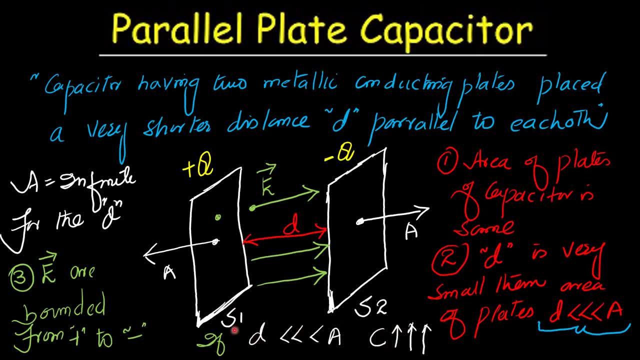 which mean that capacitance is inversely proportional to the distance between the parallel plate, Where, as if area of the plate is greater, capacitance will be greater. which mean that capacitance is directly proportional to the area of the parallel plate present in parallel plate capacitor. 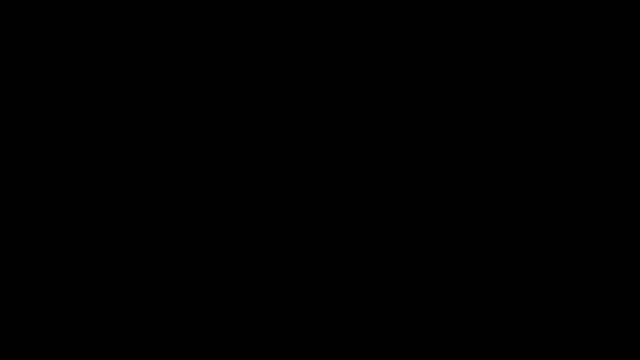 Now this student important question here appear is that how a parallel plate capacitor, how parallel plate capacitor, parallel plate capacitor stored charges? How is it possible for parallel plate to store charges, since you know that parallel plate capacitor consist of two plates and these plates are placed parallel to each other? suppose that. 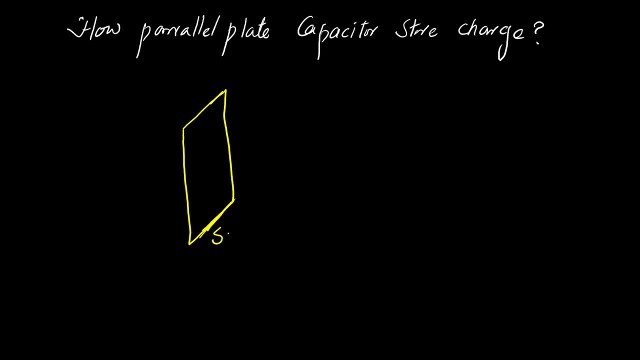 this is plate S1. the area of the plates are in parallel plate capacitor is same. So the dimension of the parallel plates in parallel capacitor, parallel plate capacitor will be same. So this suppose that this is conducting S2 plate of the parallel plate capacitor. 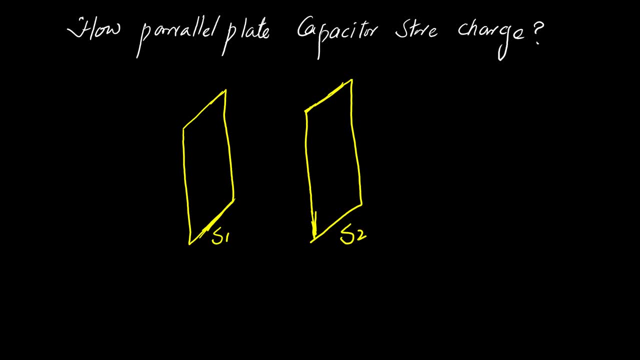 So in this situation, both the conducting plates are. they have a no charge in order to charge these parallel plate capacitors. parallel plates, basically, they are make. they are connected with a power supply. Usually they are connected with a dc power source. suppose this is a dc power source. 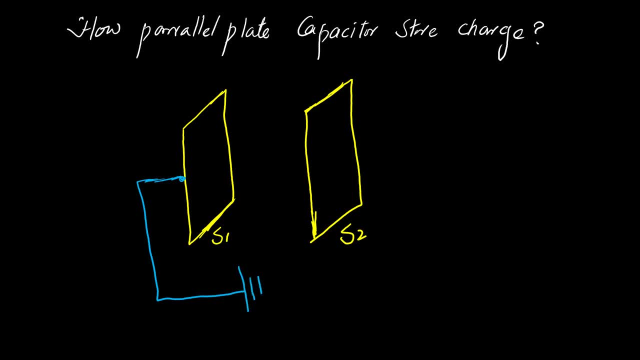 or dc battery and with this these two parallel plates are connected. So now, when these parallel plates are connected with a dc power source, these parallel plate act as a capacitor, Since the potential difference Is created due to positive and negative terminal of the dc power source and the role of a positive 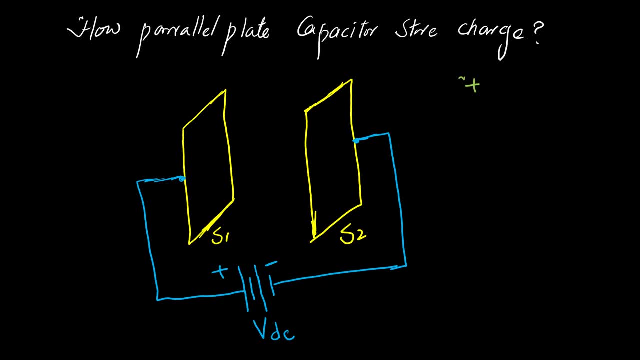 terminal is. the role of a positive terminal is to pull electron toward itself, pull electron toward itself, whereas negative terminal push electron, push electrons away from itself. So now, So The electron will move from parallel plate S1 toward the positive terminal, Like this: 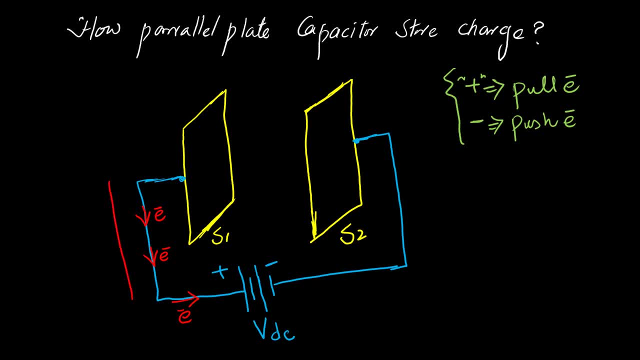 So whenever electron move from positive terminal, from plate S1, toward the positive terminal There will be, They will leave positive charge behind on the surface of the plate S1, like this, Since you know that charges reside on the surface of the conducting metal or plate. 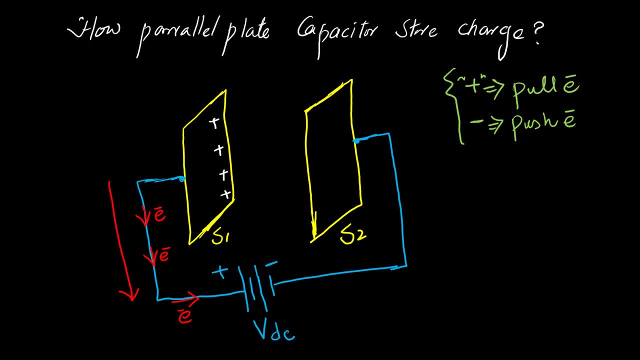 So, whenever the charges, electrons move from the surface, they will leave. They will leave positively positive charge and these positive charge will be present at the surface of the parallel plate capacitor and where- as since you know that the negative terminal- basically push electron away from itself- 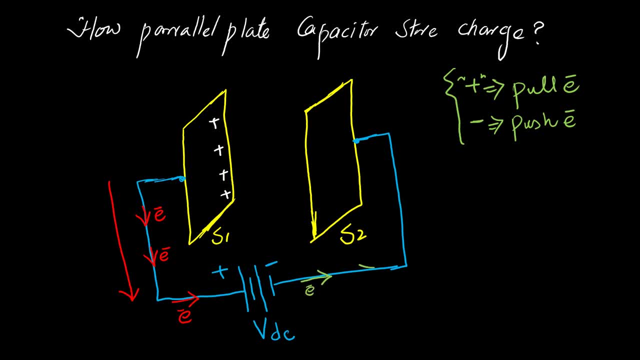 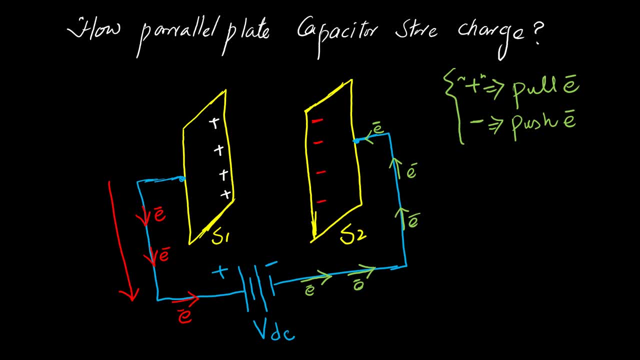 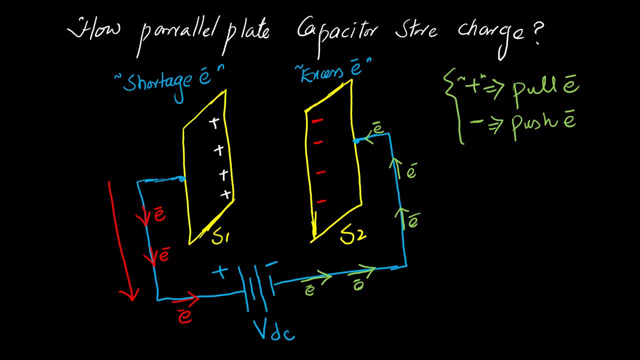 will be two types of electric field present between s1 plate and s2 plate. one electric field will be from due to a positive charge and it will be from positive to charge toward a negative charge. since you know that electric field of line travel from positive charge toward negative charge, are they? 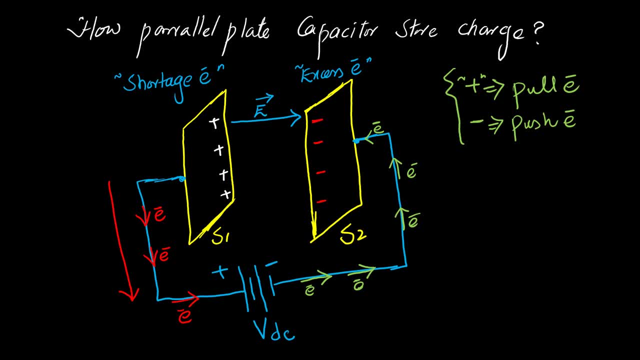 are from positive charge to negative charge, and let's say it is E1. so, like this, uniform electric field of line from positive charge to negative charge will be like this: now there will be another electric field and that electric field will be generated by a negative charge. since you know that the direction 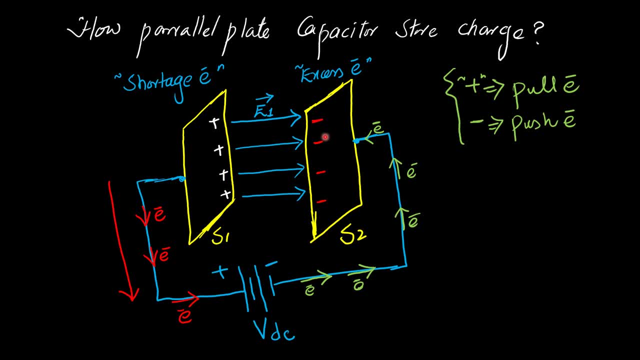 of electric field of lines are basically toward the negative charge. so these negative charge will have electric field of line but they will be toward this negative charge and they will be like this, toward negative charge. and let's say we say these electric field of line, set this Electric field of line as E 2. 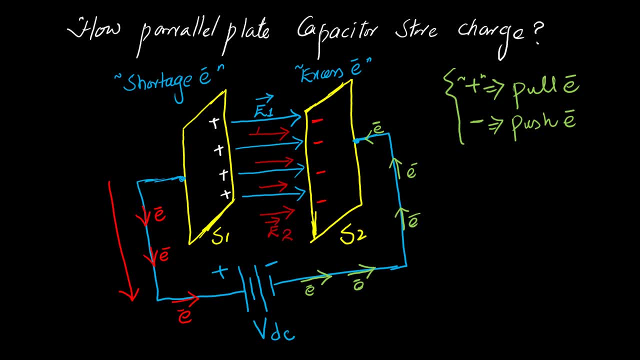 so the students total electric field generated in parallel plate capacitor will be: E is equal to nut. electric field in at will be due to electric field generated by a positive charge plus electric field generated by a negative charge. So this is a net electric field present in a parallel plate capacitors. 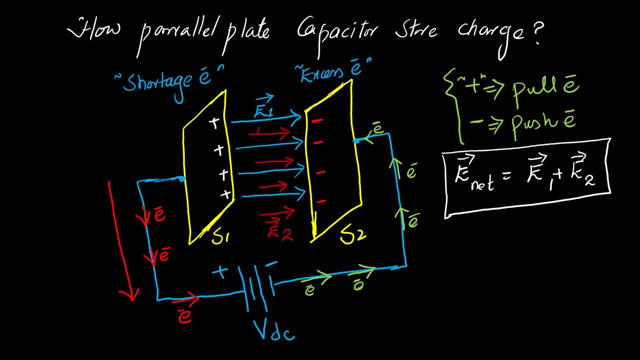 now these students, as you know that whenever there is applied electric potential, this electric potential generate charges on the surface of the plates and these there, these discharges which are present at the surface of parallel plate, have a potential difference between them, and that potential difference depend on the number of charges stored at the surface. 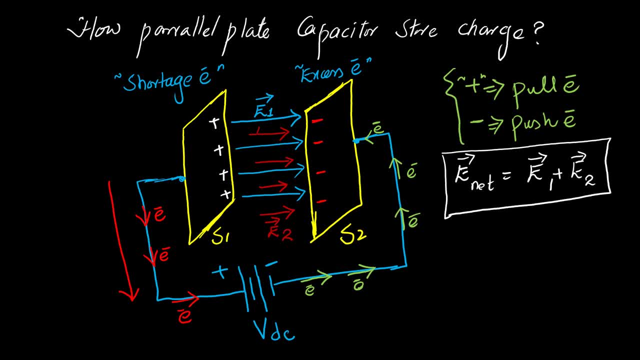 of plate, which mean that the capacitance, the, the charges, basically, are directly proportional to the potential difference. so charges stored on a parallel plate are directly proportional to the potential difference present between the plates of the charges. so due to this, as you know, that we can open this equation as Q is equal to C, 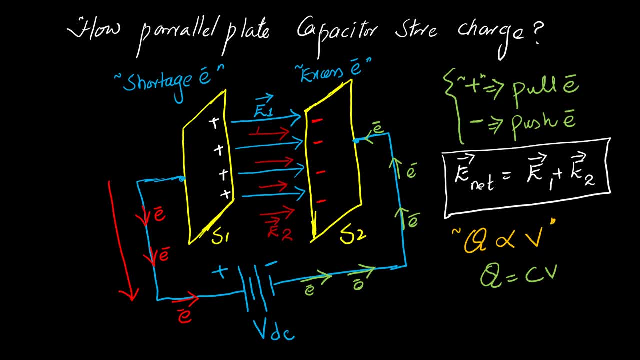 into VC the constant of proper constant proportionality, which is a capacitance of capacitance, and the capacitance of capacitance becomes C, is equal to Q divided by V. it is a ratio of charge stored in a capacitance divided by a potential difference. let's say it as equation number one now. 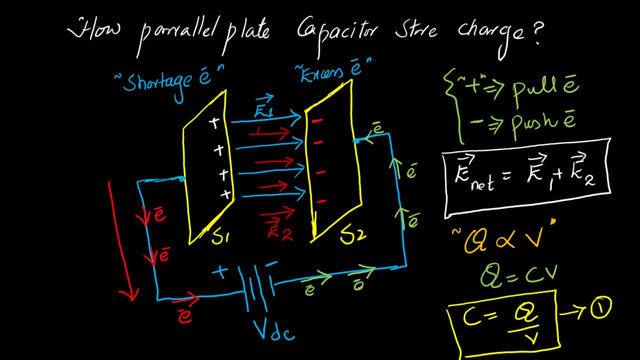 let us calculate the capacitance of a parallel plate capacitor, since you know that, in general, the equation for capacitance is: C is equal to Q divided by V, and as you know that potential difference, V is equal to E into D. E dot D étais a. 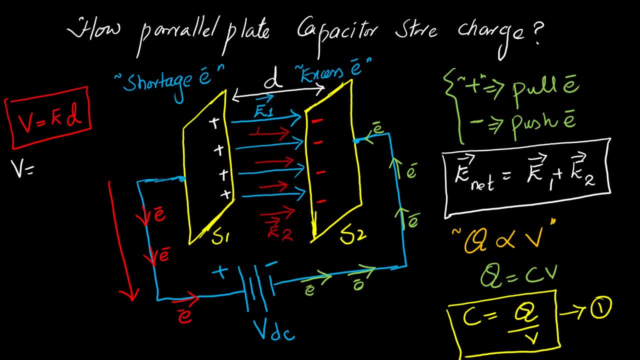 but a constant of potential difference equal to lava, V, d, d a, e1 electric field due to a positive charge plus e2 electric field due to negative charge into dd is, which is a distance between the two parallel plates, and we say this as equation number two. 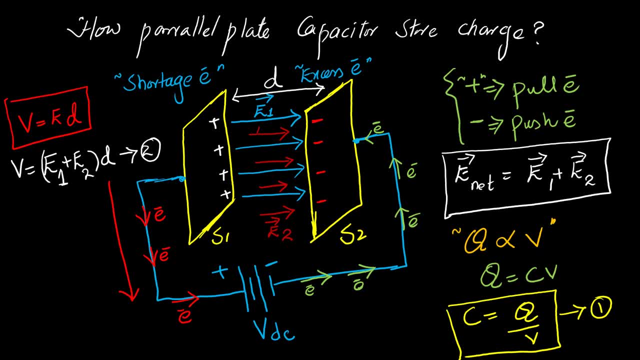 now you know that the electric field, for a electric field in a sheet, in an infinite sheet, is equal to e, is equal to e, is equal to sigma divided by two epsilon naught, whereas the sigma is basically, it is a surface charge density which is basically charged divided by area. 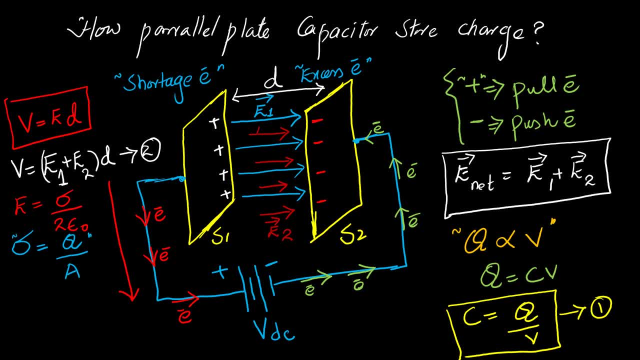 so charge on the plate divided by an area is the surface charge density. so basically we can this suppose this is equation number three. so basically we can incorporate the equation number four in equation number three and we can get that electric field intensity e is equal to if we put the value 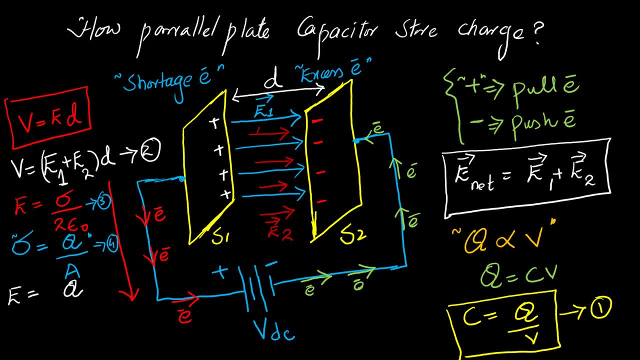 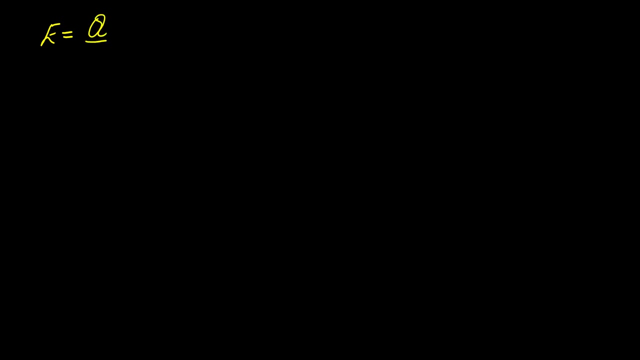 of sigma, then electric field intensity will be q divided by two. epsilon naught into a, so we can say this as equation number five. so now, since electric field intensity become, e is equal to q divided by two. epsilon naught a for an infinite plan sheet. then, as you know that there are in parallel plate capacitor there are two sheets. so the net electric 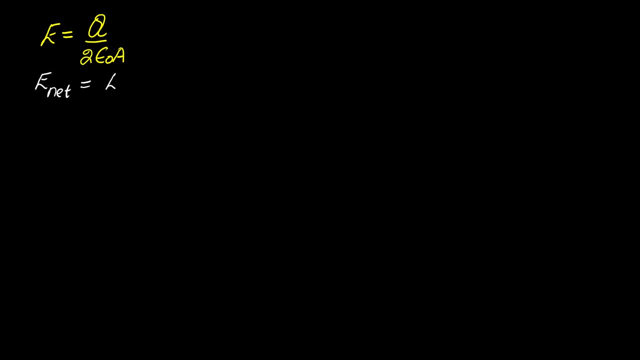 field of intensity is equal to e1, plus the electric field intensity due to a positive charge and e2. so then the net electric field of intensity become if we put the value of electric field intensity in them in. in suppose this is equation number six. in equation number six then we get q. 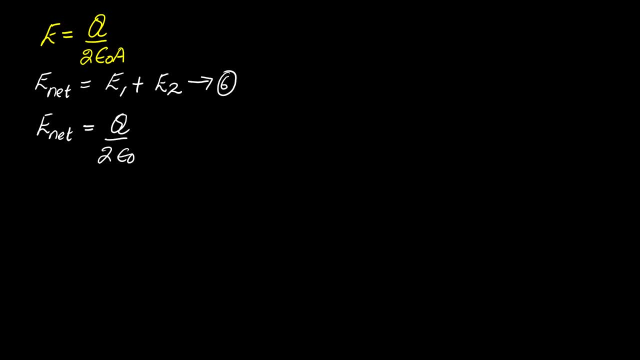 divided by epsilon a plus q divided by two epsilon a. so this equation will become check when writing the equation number four in equation number six, so this equation will become: e net is equal to 2q. 2 q divided by 2 epsilon into a a2 will cancel with 2 and that way it will not call bought would cancel. 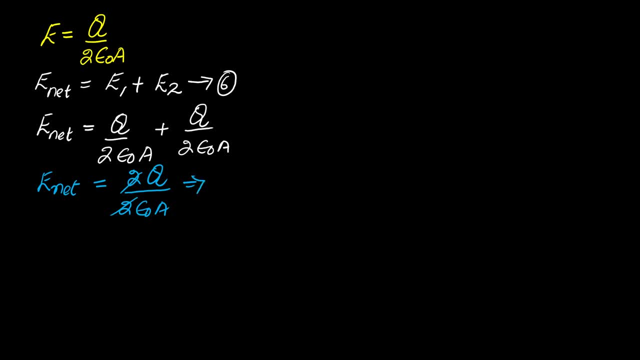 as well as being a two spirit point Dravet which would killed by two epsilon. so what called 又是 neutral line, e2, net current line of E0 z Scott, the one that D B is also interesting. and we can get net electric field of intensity as q divided by epsilon naught into a. so this will be. 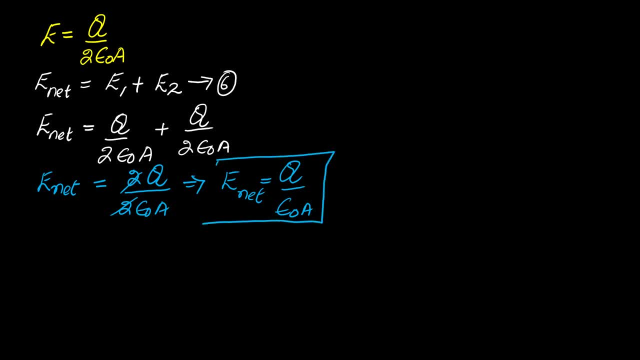 electric field of intensity between the two parallel plates of a parallel plate capacitor, and let's say that this is equation number seven. now, district, let us calculate a capacitance of a parallel plate capacitor, since you know that capacitance is equal to q divided by v. v is a potential difference and we know that a potential 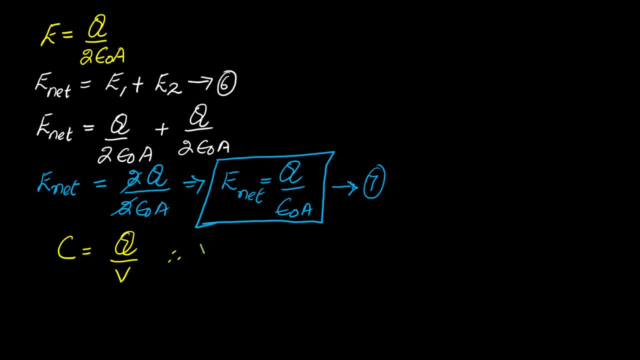 difference. v is equal to electric field intensity between the plate of capacitor into d, the spacing between the plates of the capacitor. so we can get net electric field of intensity as q divided by capacitor. so v is equal to e into d, so we can put the value of v in the equation of capacitance. 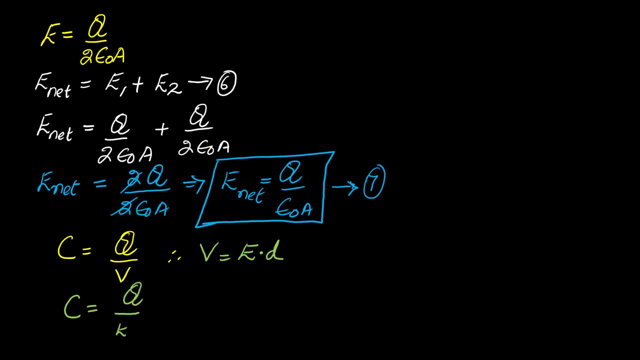 q divided by e into d. suppose that this is equation number eight. now put equation eight, eq 7 in equation 8. we basically then we get that capacitance c is equal to q divided by what is the value of e. as you know, that value of e is q divided by. epsilon naught a into d. now, dear student, please keep in. 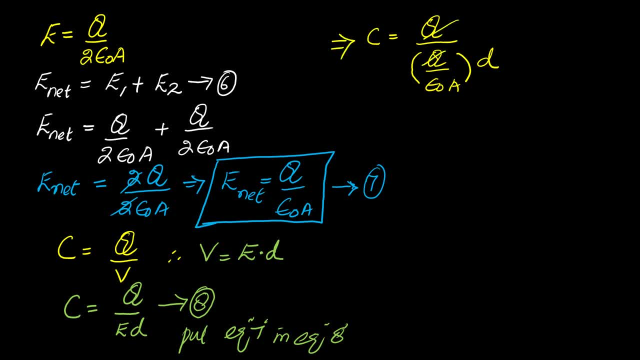 mind that q will basically cancel with q and we get a capacitance of capacitor as c is equal to 1 over d divided by epsilon naught a. if we rearrange an equation, this equation, then we can easily get that capacitance of parallel plate capacitor is equal to. 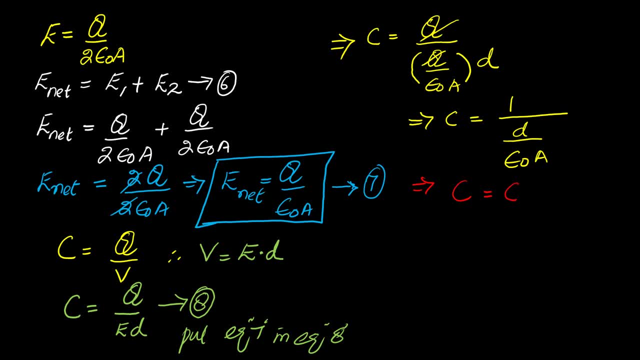 epsilon naught a divided by d. this means that a capacitance of a capacitor depends on area of a plates, area of plates and and capacitors of capacitors depend on distance between the plates. so if the area of plate is more, if the area of plate is more, the capacitance value of capacitance. 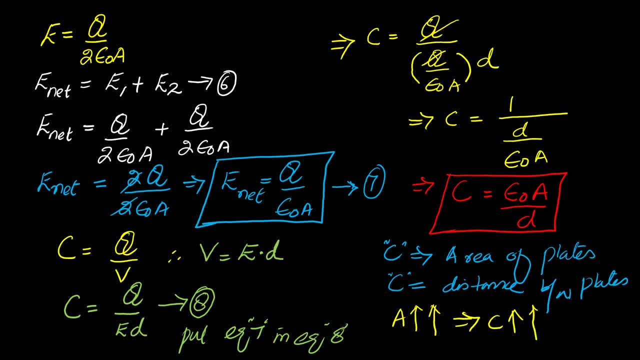 will be more, and if a distance between two parallel plate d d is more, then the capacitance will be less. this means that capacitance is directly proportional to the area of the plate and inversely proportional to the distance between the plates. greater will be the distance. 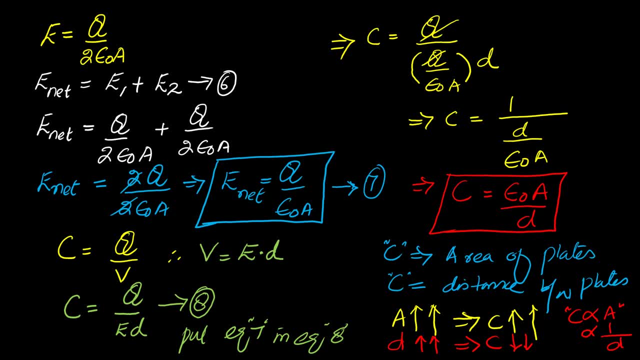 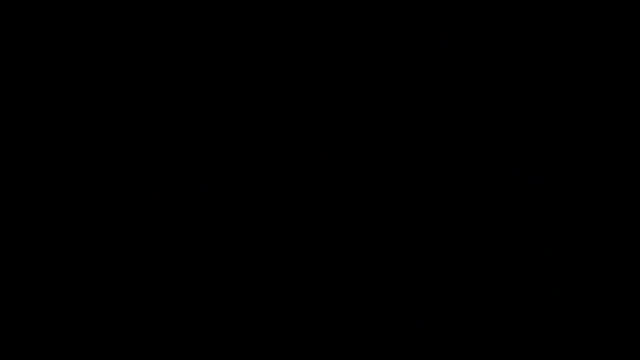 lesser will be the capacitance and lesser of the distance, greater will be the value of capacitance. now this trend. please keep in mind that for for parallel plate capacitor, it is not necessary that the conducting plates are a rectangular shape. they can be of different shape, they can be a square. 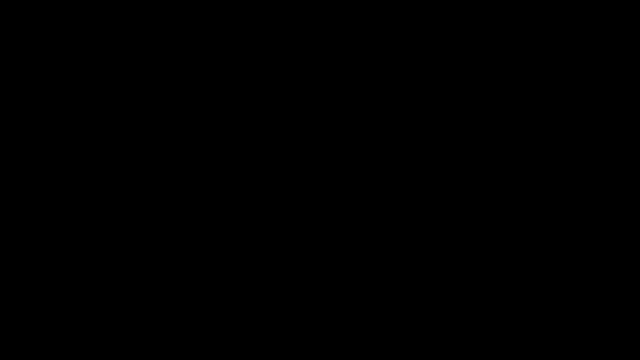 they can be circular, if they can be a circular, but the main uh uh. but the key, important point to notice here is that the area of the plates of parallel plate must be must be same and secondly, they must be placed parallel to each other. so if we have a parallel, circular, parallel, 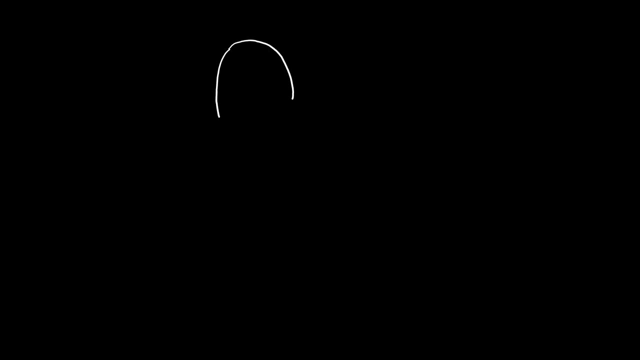 plate capacitor like this. suppose that this is a circular parallel plate. let me read out the circle, because not completely pure circle. so if we have a circular parallel plate capacitor, suppose this is a circle s1 and this is a circle, suppose s2. both the area of the circle is same. and suppose this: 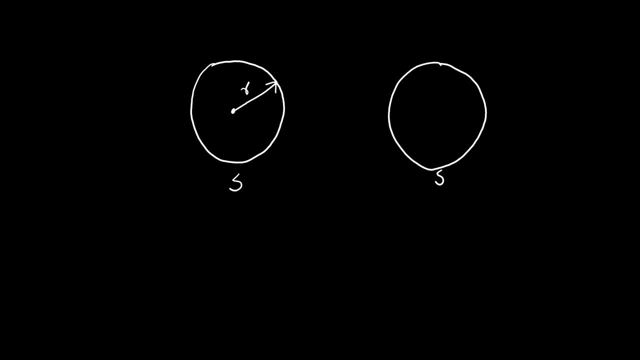 r is a radius of a circus and circle and both the radius of the plate, circular plate, of the parallel plate capacitor are same. then, and the distance between these two plates is suppose it is x. then what will be the capacitance, what will be the value of capacitance of this circular parallel? 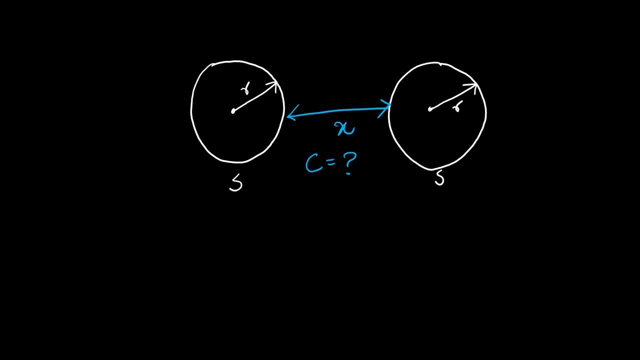 grade capacitor. how can you calculate the capacitance value for circular parallel plate capacitor, since you know that, as we have drawn the formula, capacitance for a parallel plate capacitor is equal to epsilon naught a, epsilon naught a divided by d? so now, as you know that area of a circle, area of a circle is equal to pi r square.